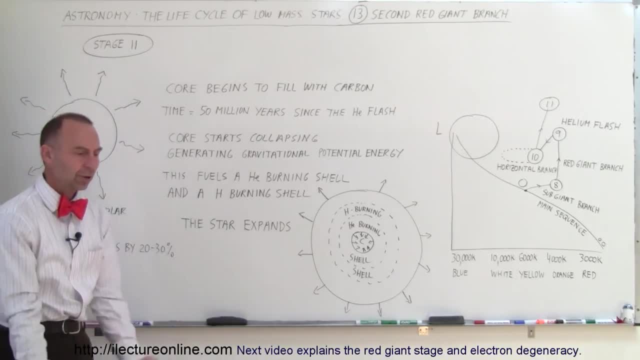 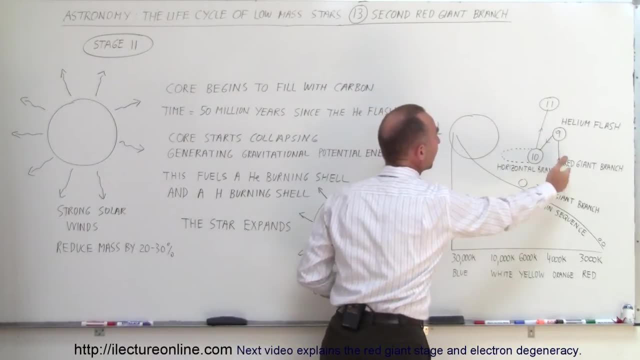 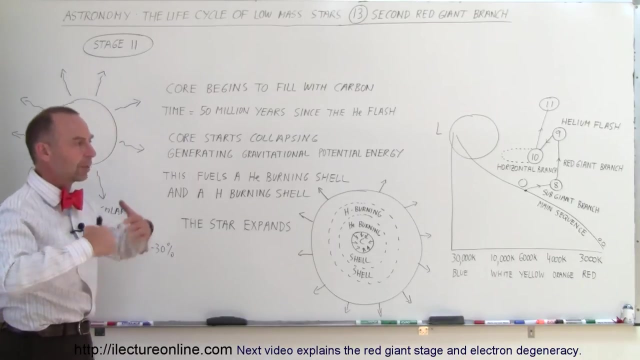 And as the star begins to expand, it becomes larger. Since the surface area becomes larger, the luminosity of the star increases and you can see how the star begins to climb back up the H-R diagram. in parallel to the first red giant branch, we now have what we would call our second red giant branch, with the 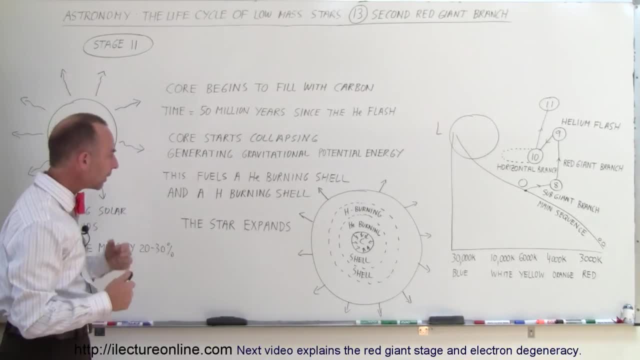 star becoming larger and larger and more luminous and more luminous. This continues to go on until the star reaches a point where the core is again going to be arrested by the repulsive force of the electrons, the electron degeneracy. But during that stage the star grows to a very, very, very large size. 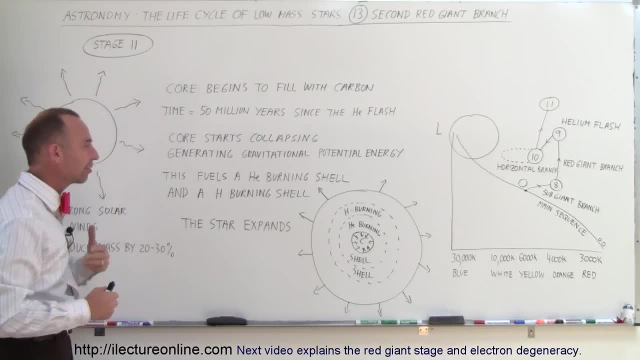 All right. And also during that period the solar winds become very strong As a red giant. and as it grows to that second red giant, what we call red giant branch stage, the solar winds really pick up and begin to carry off enormous quantities of. 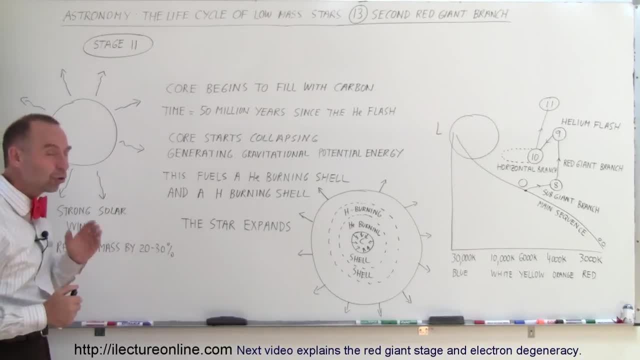 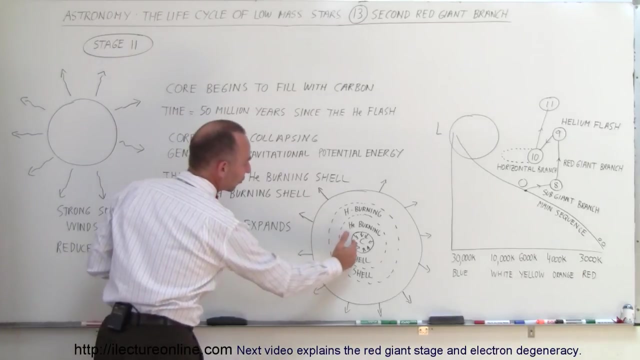 the star's mass. So the star in that stage can lose as much as 20 to 30% of its total mass by the solar winds, and not at high speeds but at very gentle speeds- just gets carried away. and of course the reason why it's able to do that is also because these 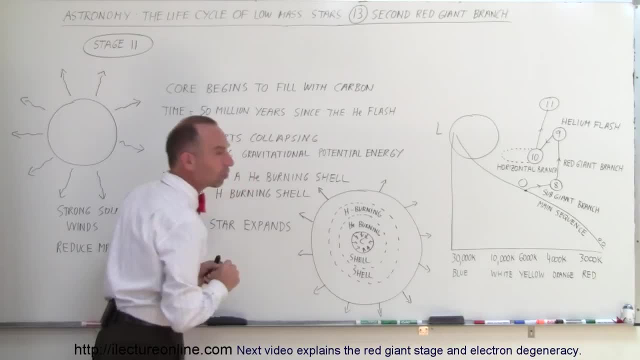 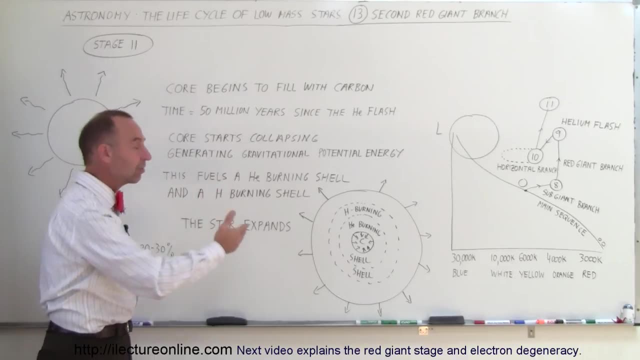 outer regions of the star are so far away from the center of the star that the gravitational forces at the very edge of the star aren't as strong, and so it doesn't take a lot of speed, a lot of velocity for the wind to carry mass away from the star. and so there we are, at the second red giant. 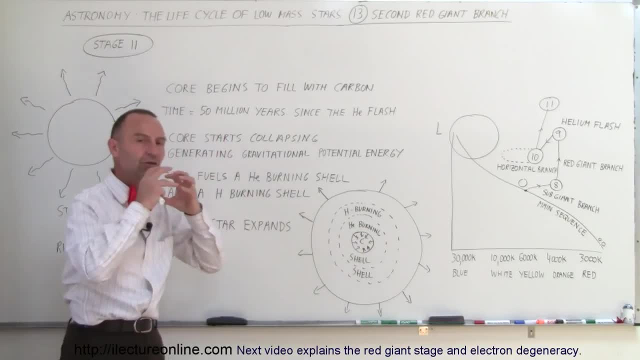 branch stage where the core begins to collapse down into a solid ball of carbon. it turns out most of the carbon that we have in our bodies comes from these places right there. but how it gets from there to here, well, that's another story for another video at some other time. 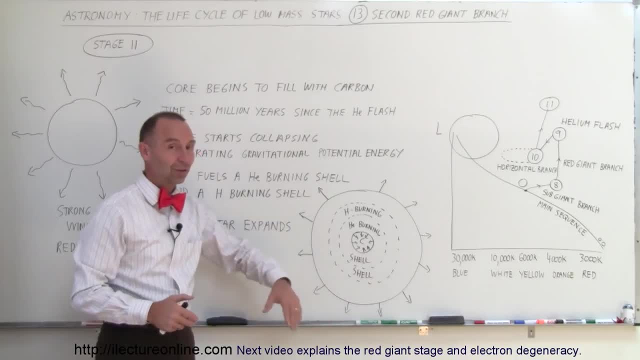 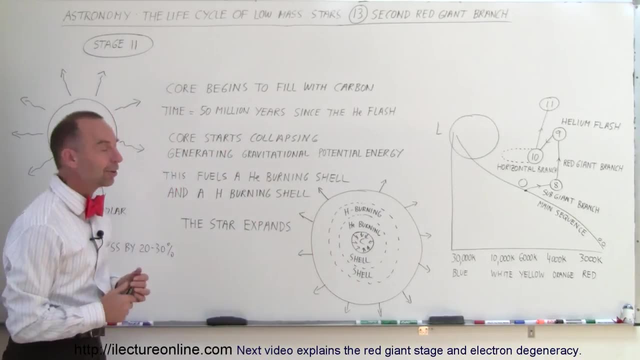 but it's just interesting that most of the carbon in the world- or i should say all of the carbon in the world- comes from the center of stars and somehow it went from here to the earth and where we have it in our bodies. but i'll leave you wondering about how that happens until we make 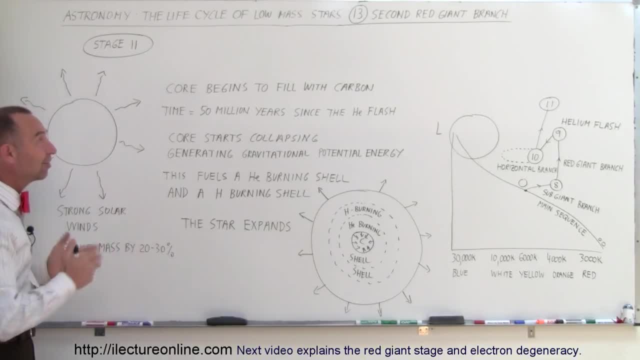 the video to show you how that that occurs. but anyway, that is what we call the second red giant branch stage, and so now we're set up to see what happens. at that point, some very interesting things are going to happen to the star before it comes to its final demise as a white dwarf.